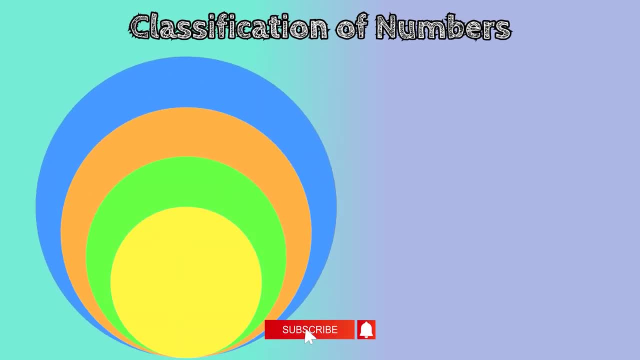 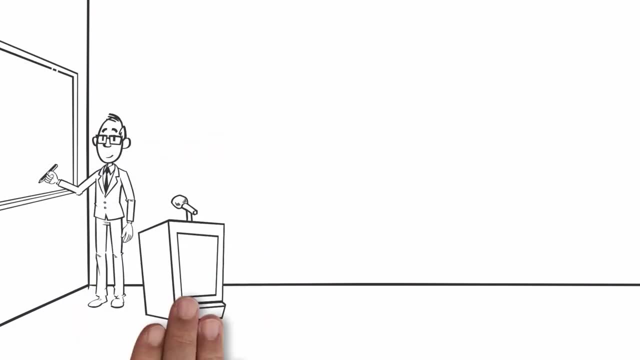 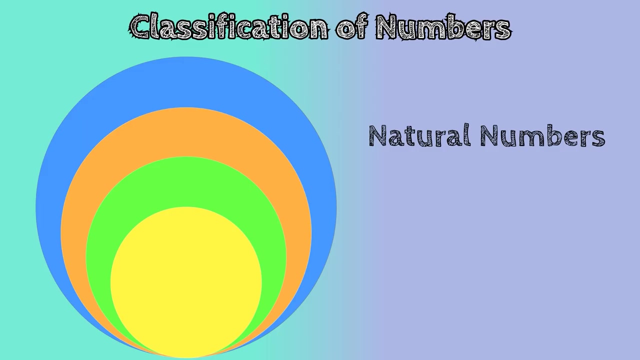 types of numbers that exist in the world of math. The first set of numbers are natural numbers. Think of natural numbers as counting numbers. When we were really young and first started school, we learned how to count. The numbers we learned in kinder were 1,, 2,, 3,, 4,, 5,, 6,, 7,, 8, and so on. 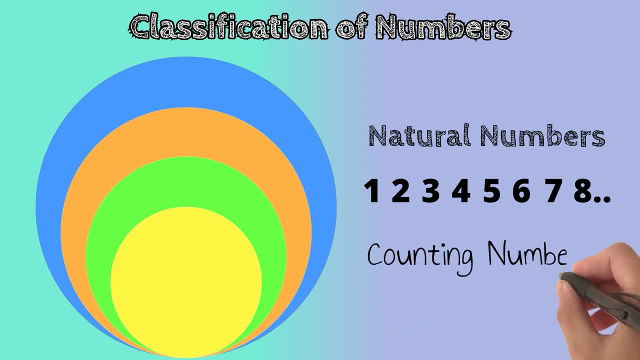 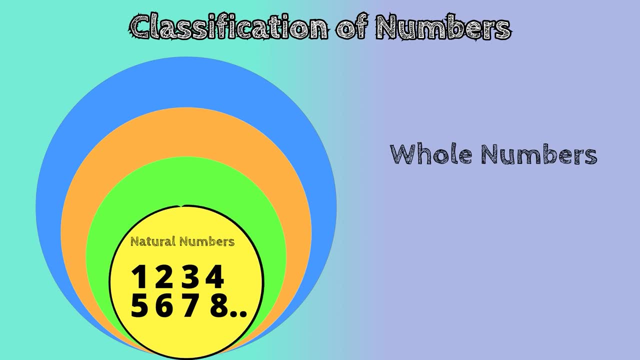 You can think of natural numbers as counting numbers. The next set of numbers we have are whole numbers. Whole numbers include all natural numbers such as 1,, 2,, 3,, 4,, 5, and so on, but they also include the digit 0. Think of whole numbers being different from natural. 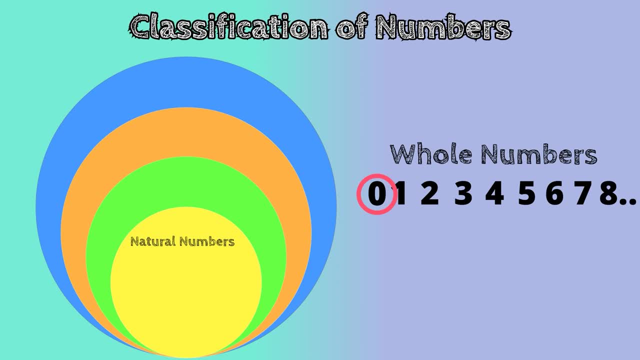 numbers, since they include the number 0 where natural numbers do not. And how different life would be without the number 0?? After whole numbers, we have integers. Integers include all natural numbers, such as 1,, 2,, 3,, 4,, 5,, 6, and so on. They also include all whole numbers. 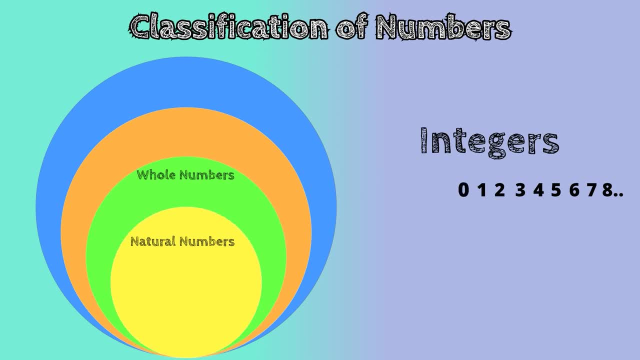 so we will add the zero to our list. But they also include negative numbers. So to the left of our set of numbers we will add negative 1, negative 2, negative 3,, negative 4, and so on. You�ve probably seen negative numbers in temperature change or in marking certain. 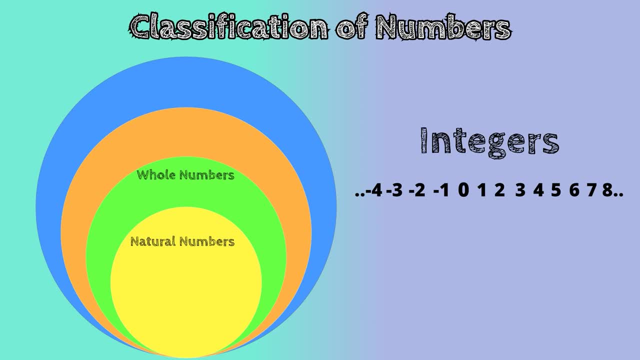 locations such as below sea level. Integers are different from natural and whole numbers in that they include negative numbers. Things You Need to Know About Natural Numbers learning about are rational numbers. Rational numbers include all natural numbers, such as 1,, 2,, 3,, 4,, 5, and so on. They also include whole numbers, So let's go ahead and add a 0 to the. 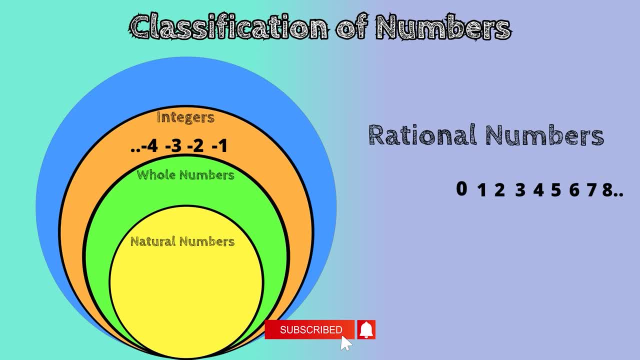 left of 1.. They include all integers, So let's add negative 1, negative 2, negative 3, negative 4, and so on. But now we will add fractions, decimals and percents. Rational numbers include a mixture of fractional parts and whole numbers, So let's add a future example: Negative. 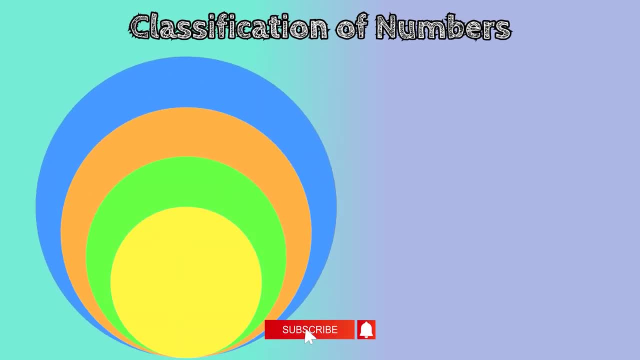 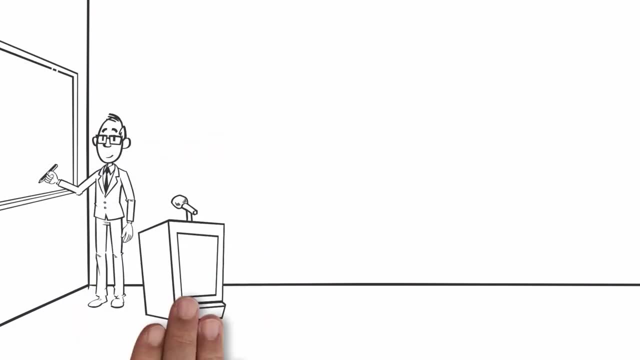 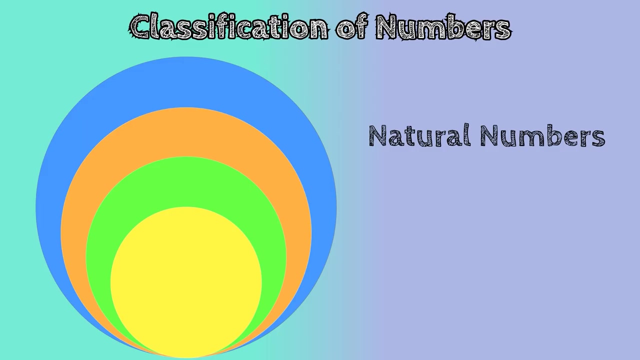 types of numbers that exist in the world of math. The first set of numbers are natural numbers. Think of natural numbers as counting numbers. When we were really young and first started school, we learned how to count. The numbers we learned in kinder were 1,, 2,, 3,, 4,, 5,, 6,, 7,, 8, and so on. 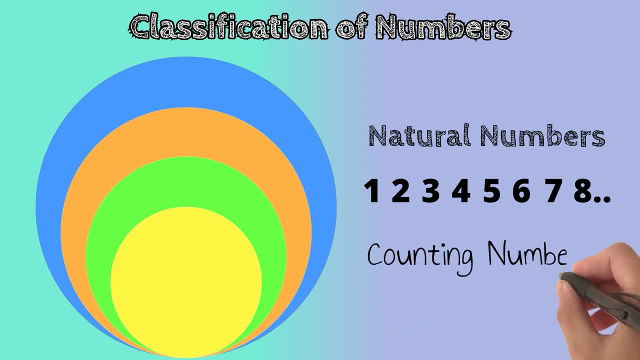 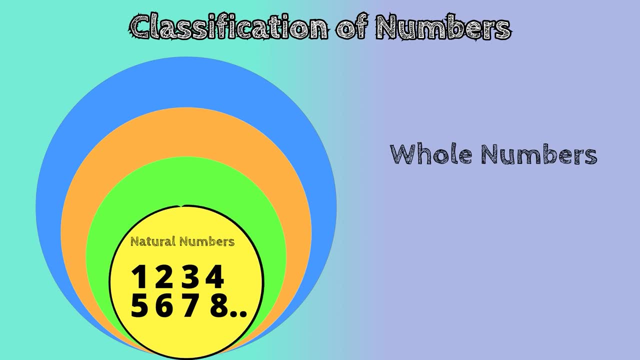 You can think of natural numbers as counting numbers. The next set of numbers we have are whole numbers. Whole numbers include all natural numbers such as 1,, 2,, 3,, 4,, 5, and so on, but they also include the digit 0. Think of whole numbers being different from natural. 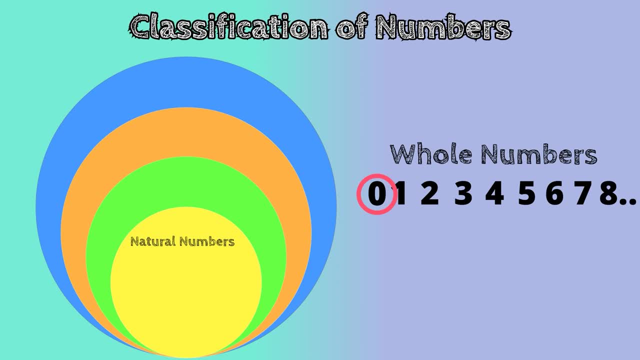 numbers, since they include the number 0 where natural numbers do not. And how different life would be without the number 0?? After whole numbers, we have integers. Integers include all natural numbers, such as 1,, 2,, 3,, 4,, 5,, 6, and so on. They also include all whole numbers. 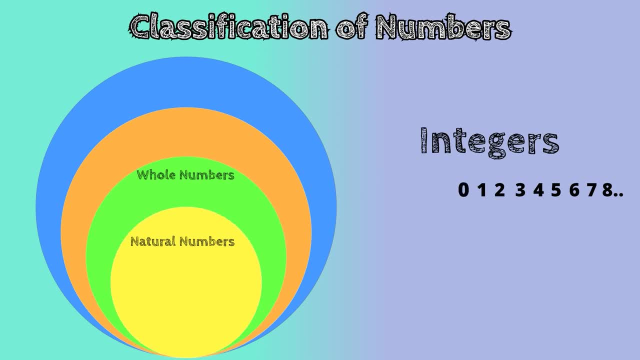 so we will add the 0 to our list. But they also include negative numbers. So to the left of our set of numbers we will add negative 1,, negative 2,, negative 3,, negative 4, and so on. You've probably seen negative numbers in temperature change or in marking certain. 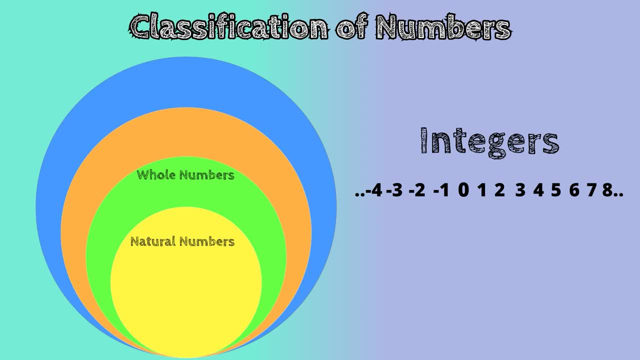 locations such as below sea level. Integers are different from natural and whole numbers in that they include negative numbers. The last group we will be learning is called numbers. Rational numbers include all natural numbers such as 1,, 2,, 3,, 4,, 5, and so on. They also 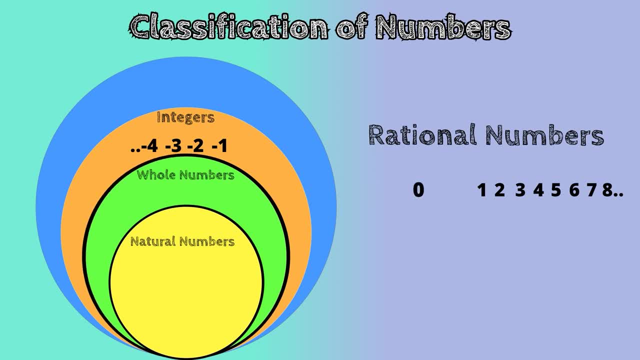 include whole numbers, so let's go ahead and add a 0 to the left of 1.. They include all integers, so let's add negative 1, negative 2, negative 3,, negative 4, and so on. But now we will add fractions, decimals and percents. 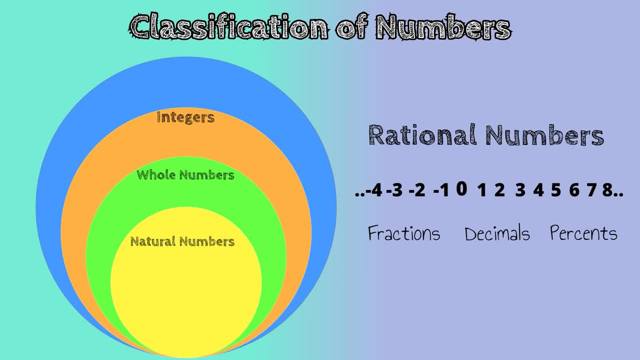 Rational numbers include a mixture of fractional parts and whole numbers, So let's add a few to our example. Negative 1 and five tenths, negative three fourths and 12 over 8 are rational numbers- 16. Rational numbers also include repeating decimals. For example, 4 over 9 is a repeating. 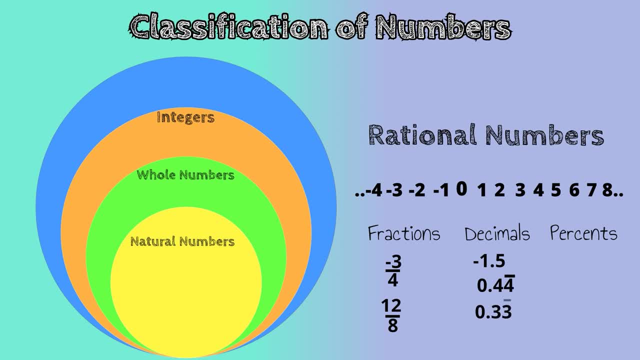 decimal 17.. 1 over 3 would also be a repeating decimal. 18.. правда 4 over 7 is the same as a repeating decimal. 24 over 3 would also be a repeating decimal. repeating decimal. Lastly, we have percentages. A percent, such as 125% or 85%, is also considered. 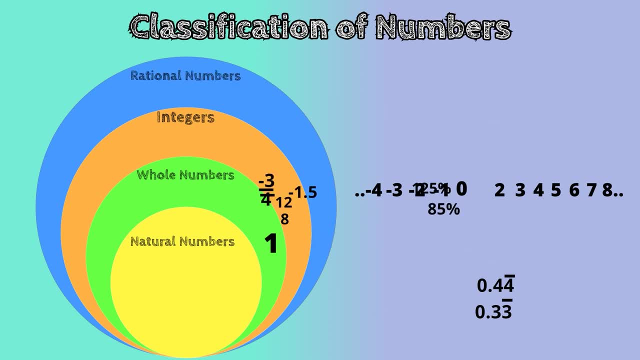 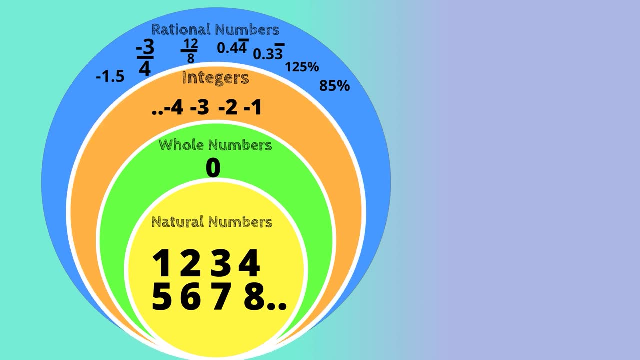 a rational number. So, if we look at our diagram, all natural numbers, whole numbers and integers are rational numbers, since they're inside of the rational number circle. Next we have integers. All natural and whole numbers are integers, since they're inside of the integer ring. 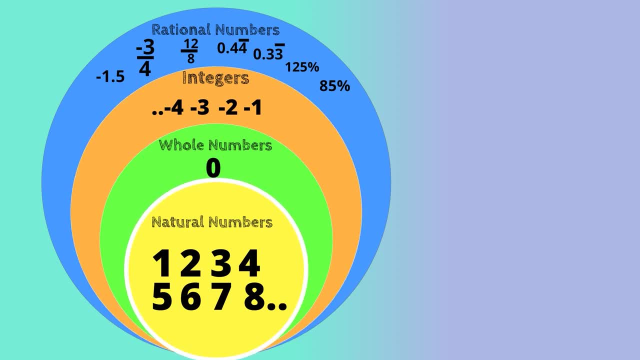 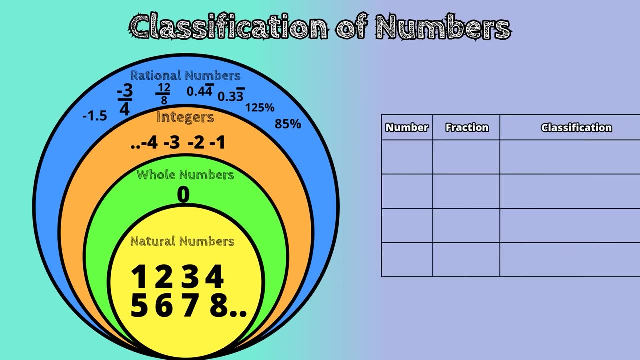 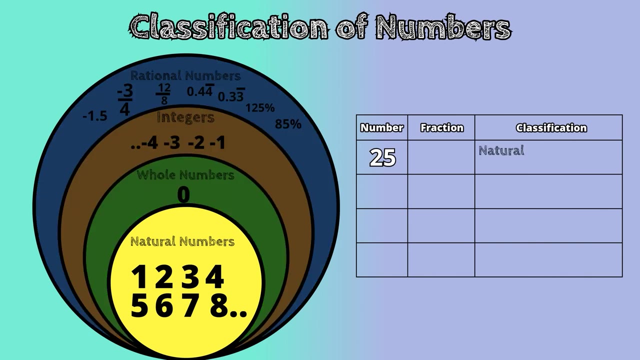 Then we have whole numbers. All natural numbers are whole numbers since they're inside the whole number ring. So let's try to classify a few numbers. Let's say we have the number 25.. The number 25 can be classified as a natural number or counting number as a whole number. 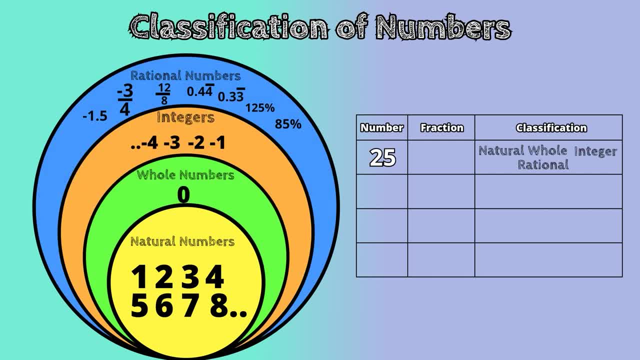 as an integer And as a rational number, since it can be expressed as a fraction: 25 over 1.. The number negative 9 can be classified as an integer and a rational number, since it can be expressed as a fraction, such as negative 9 over 1.. However, it cannot be classified as a natural. 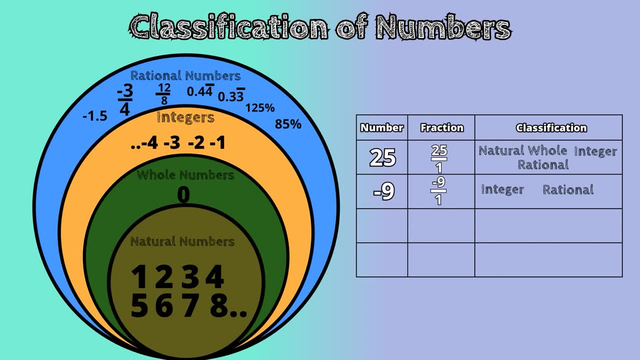 number or whole number, because these groups do not include negatives. The number 2 and 54 hundreds and positives are considered rational numbers, since they're inside of the rational number. We twist them by specific weightings and numbers. Integers are classified only as a rational number, since they're inside of the rational. 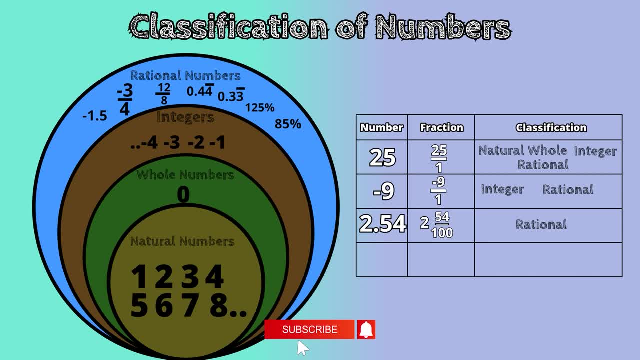 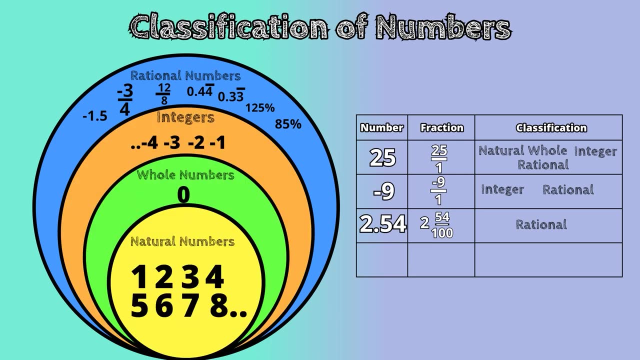 number. Integers do not include decimals, only the digit 0,. positives and negatives, Whole numbers also do not include fractions and decimals, And natural numbers do not include decimals and fractions. Lastly, how do we classify the number 0?? 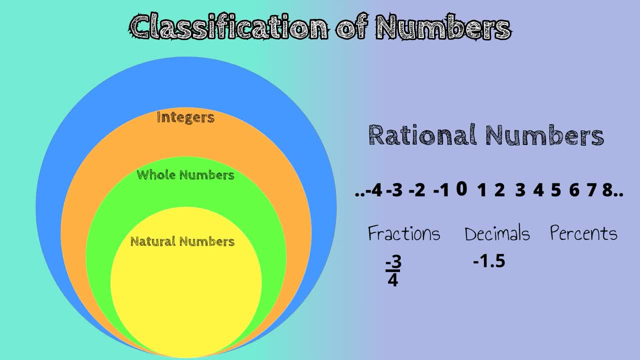 1 and 5, tenths, negative 3, fourths and 12 over 8 are all rational numbers. Rational numbers also include repeating decimals. For example, 4 over 9, is the same as a repeating decimal. 1 over 3 would also be a repeating decimal. 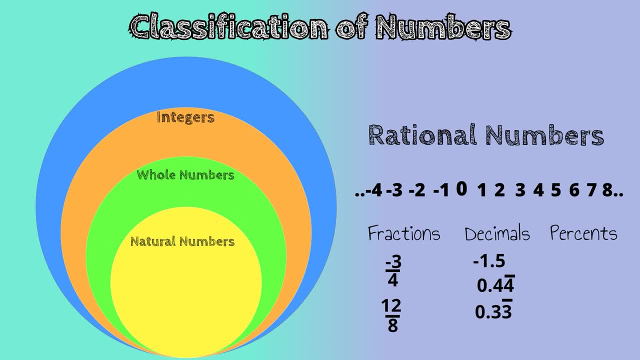 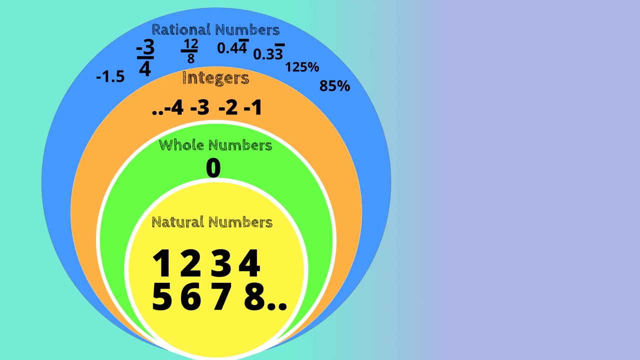 Lastly, we have percentages. A percent, such as 125 percent or 85 percent is also considered a rational number. So, if we look at our diagram, all natural numbers, whole numbers and integers are rational numbers, since they are inside of the rational numbers. 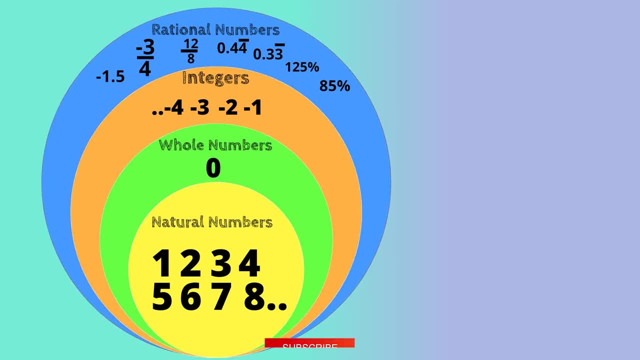 Next we have integers. All natural and whole numbers are integers, since they are inside of the integer ring. Then we have whole numbers- All natural numbers are whole numbers, since they are inside the whole number ring. So let's try to classify a few numbers. Let's say we have the 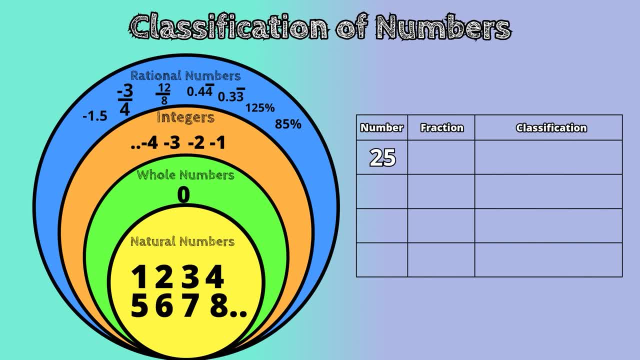 number 25.. The number 25 can be classified as a natural number or countable. So let's say we have a counting number as a whole number, as an integer and as a rational number, since it can be expressed as a fraction: 25 over 1.. The number negative 9 can be classified as an integer and a. 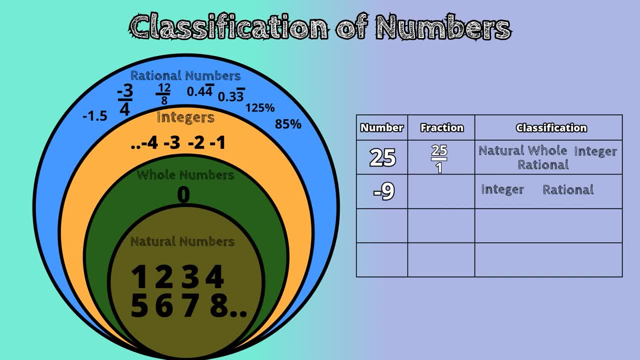 rational number, since it can be expressed as a fraction, such as negative 9 over 1.. However, it cannot be classified as a natural number or whole number, because these groups do not include negatives. The number 2 and 54 hundredths would be classified only as a rational number. Integers do not include 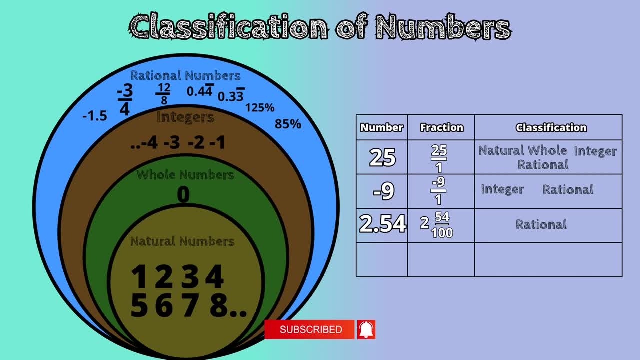 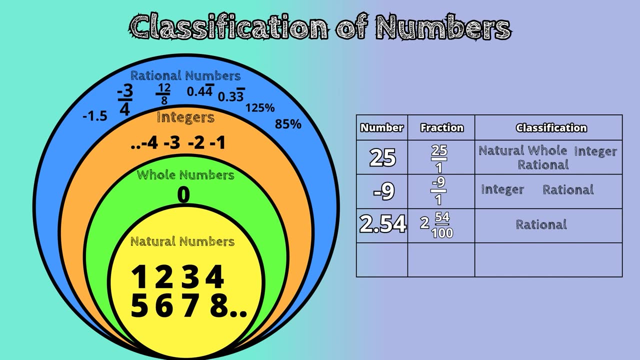 decimals, only the digit 0, positives and negatives. Whole numbers also do not include fractions and decimals and natural numbers do not include decimals and fractions. Lastly, how would we classify the number 0?? The number 0 would be classified as a rational number. 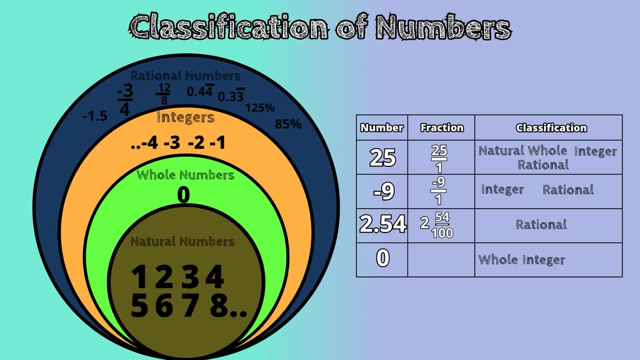 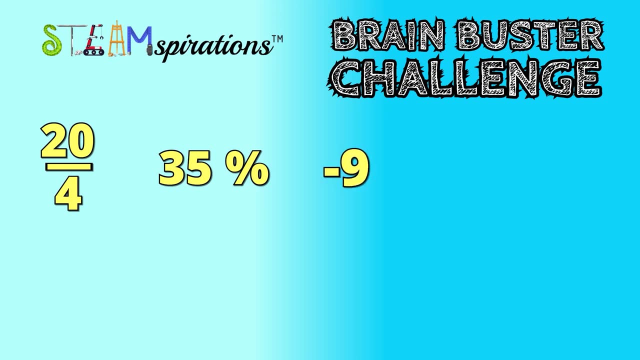 Would it be classified as a whole number, integer and rational number, because natural numbers do not include the number 0?. Here's your challenge for this video: How would you classify 20 over 4,, 35 percent negative, 9,, positive 3, and the number 1000, applying what we learned today about natural? 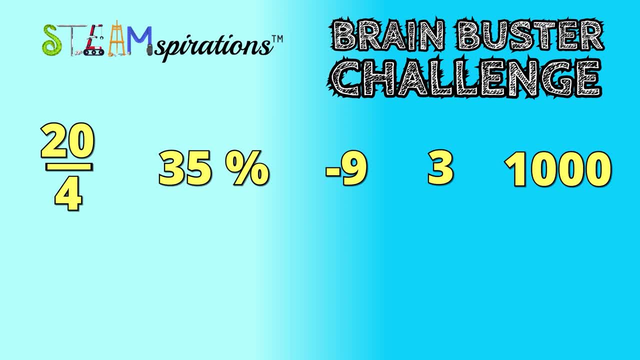 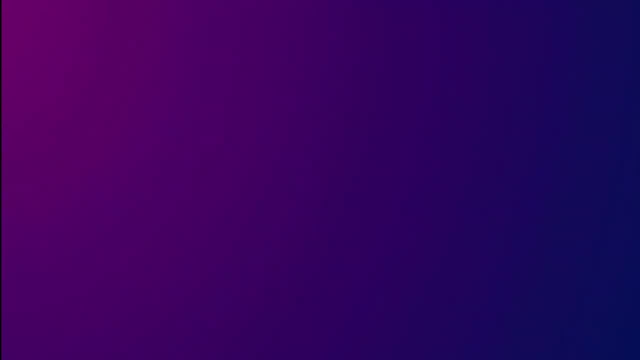 whole integers and rational numbers. So go ahead and pause the video to solve the problem and post your answer as a comment so I can get back to you. If you're looking to master various concepts in math and science, you can subscribe to our channel. Don't forget to subscribe. 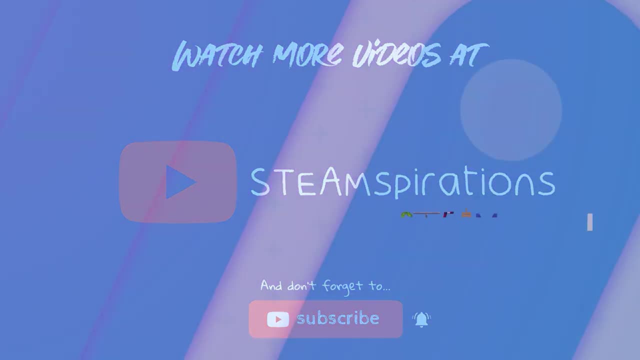 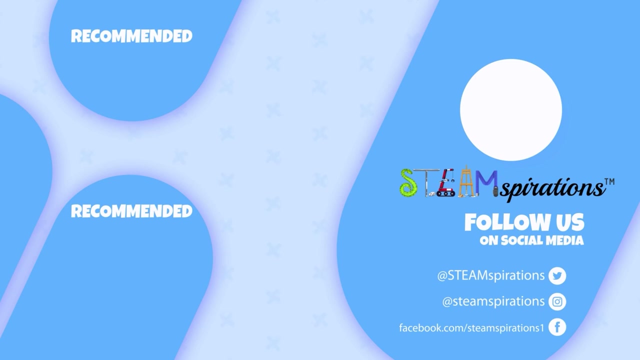 to our channel so you don't miss out on any future videos. I'll see you in the next video. 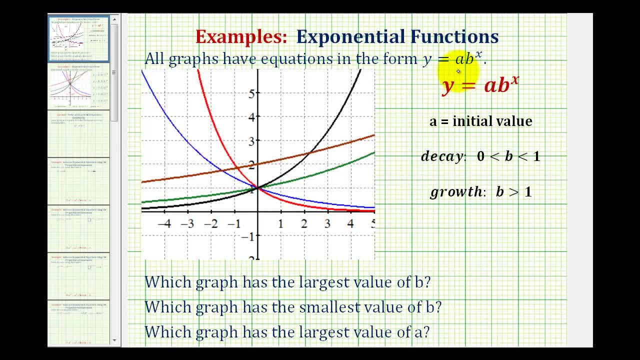 All the graphs have equations in the form: y equals a times b to the x, which means they're all exponential functions. We want to determine which graph has the largest value of b, which graph has the smallest value of b and which graph has the largest value of a. So for a. 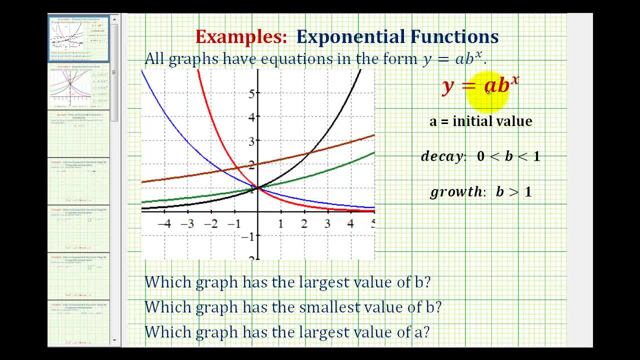 quick review. if we have an exponential function in the form y equals a times b to the x, a is called the initial value or the function value when x is equal to zero. Notice, if x is equal to zero, we would just have b to the zero, which is equal to one, so y would 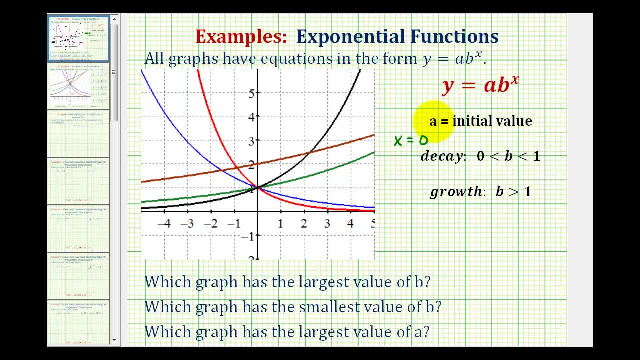 be equal to a times one. The reason it's called the initial value, though, is because a lot of times we use the variable t instead of x to represent time, and when time is equal to zero, a would be the starting amount before the exponential growth or decay starts. But